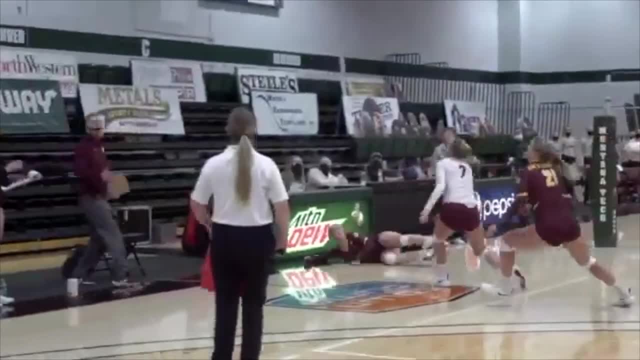 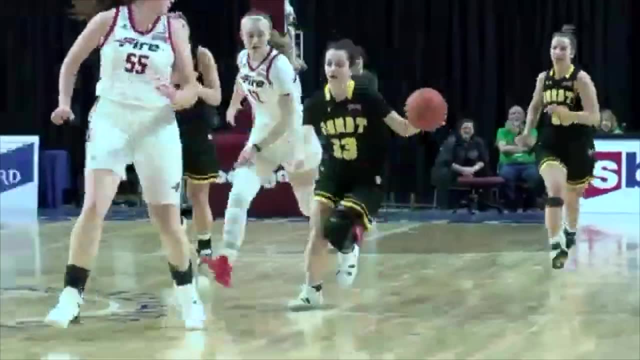 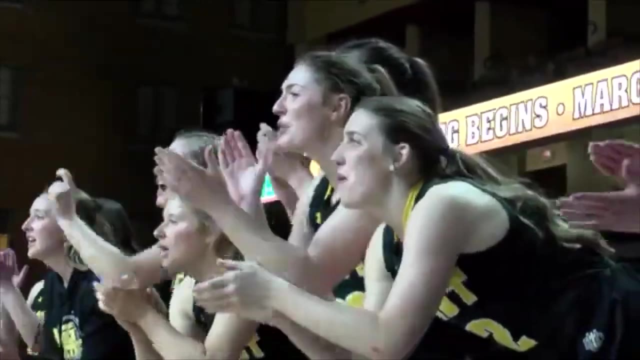 could easily play with any of the best programs in those divisions. for NCAA, It is fair to point out that NAIA schools don't get much television coverage, but the same could also be said of even the lower half of Division I. And in order to determine if NAIA is a good fit for you, 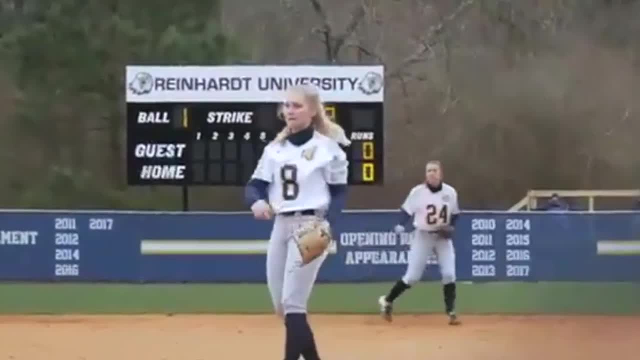 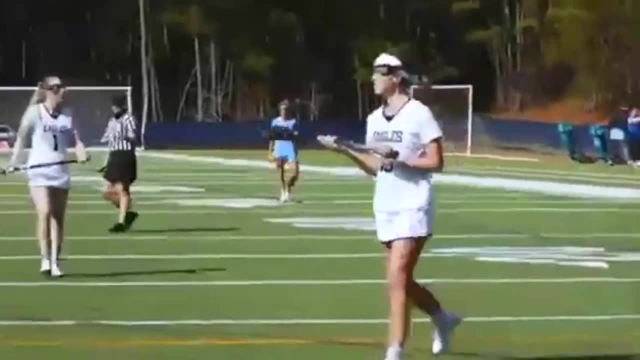 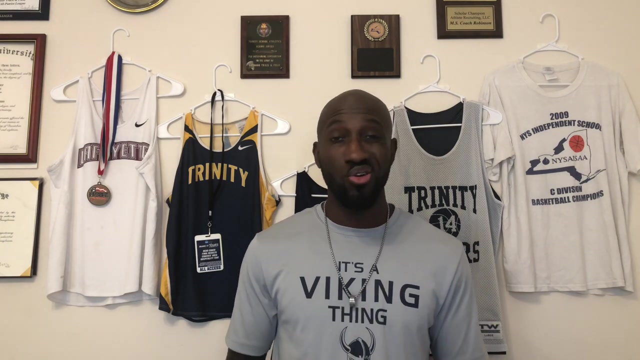 there is no blanket statement that could be made to tell every single recruit whether it is or is not, But there are a few trends that you should consider If you're a student who has a GPA that might be perhaps below the 3.5 mark, or you don't necessarily have the 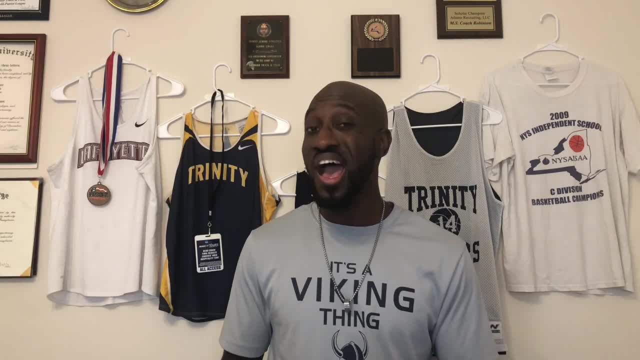 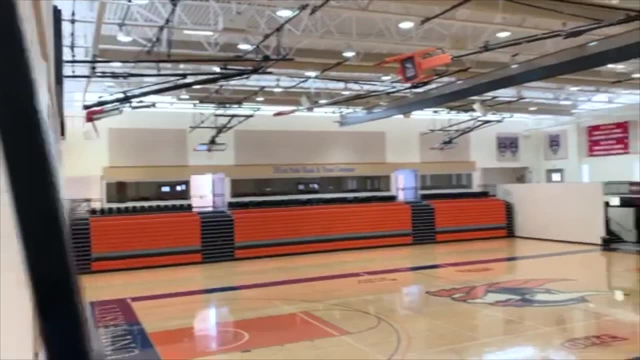 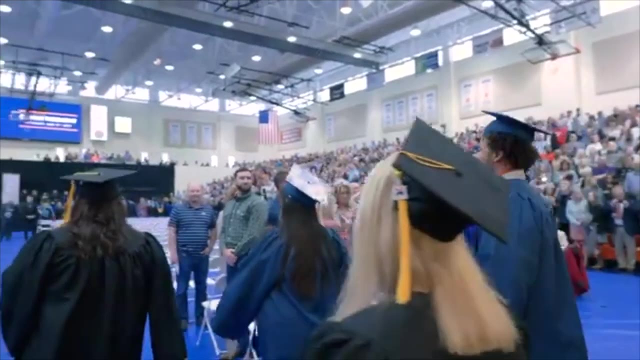 highest standardized test scores. NAIA schools might become the best option for you to find a school that values what you can offer not just athletically, but also academically. Many NAIA schools are private institutions, but their tuition costs are normally lower. on average than private Division I and Division III schools. This means that NAIA schools are often times more affordable than some other programs you might find in the NCAA. And athletically, NAIA and Division II are so incredibly similar that we could probably swap out. 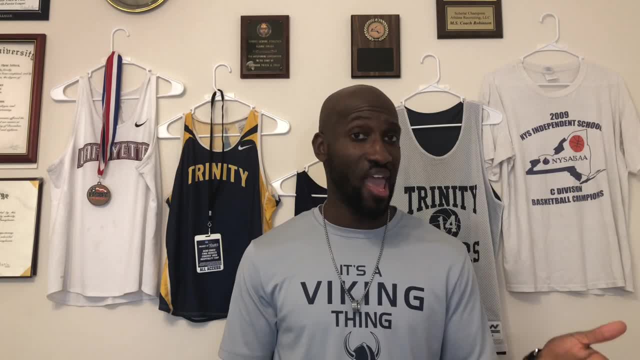 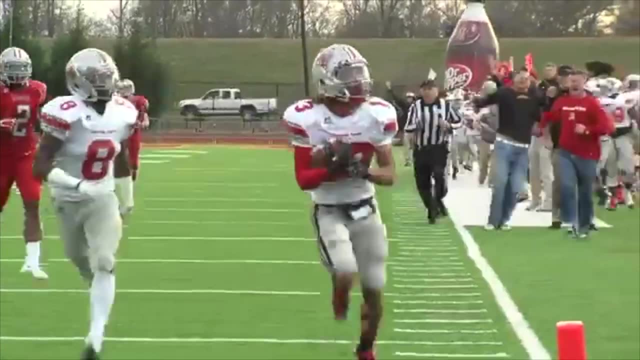 entire conferences from DII and NAIA and no one would be able to tell the difference. If you are determined to go Division I, or you have perhaps fallen in love with a Division III school, by all means you should pursue it. If you are determined to go Division I, or you have perhaps fallen in love with a Division III school, by all means you should pursue it. 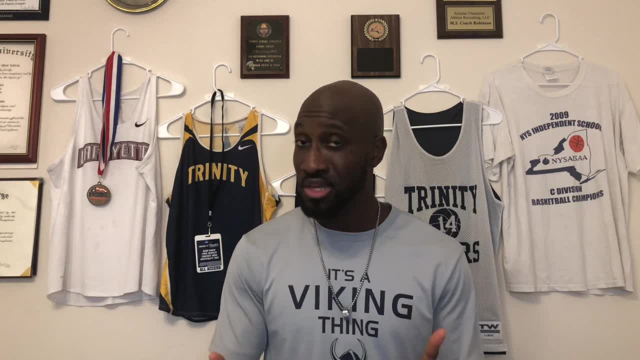 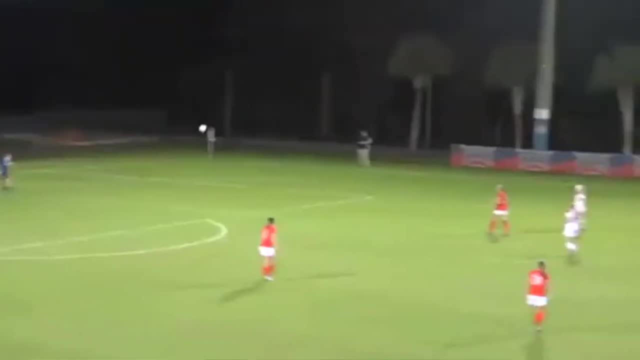 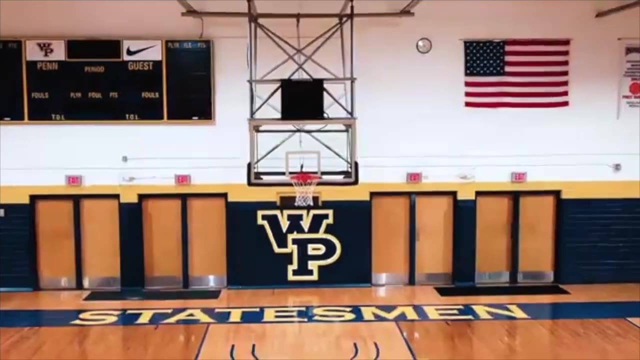 But if that is not who you are, you have nothing to lose and everything to gain by considering NAIA schools as an option. NAIA programs have different recruiting regulations than the NCAA, so you can have more conversations, take more visits and expand your recruiting options. 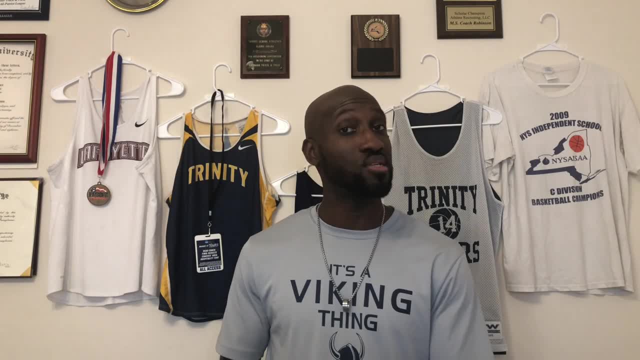 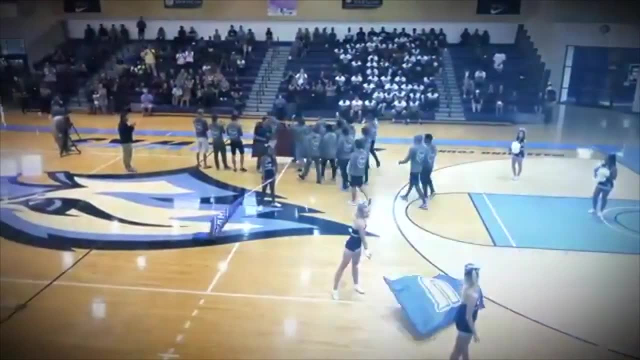 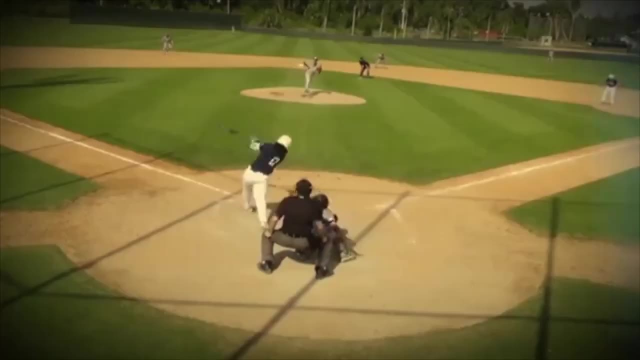 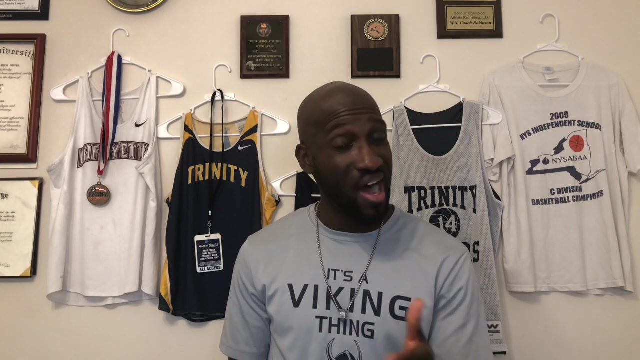 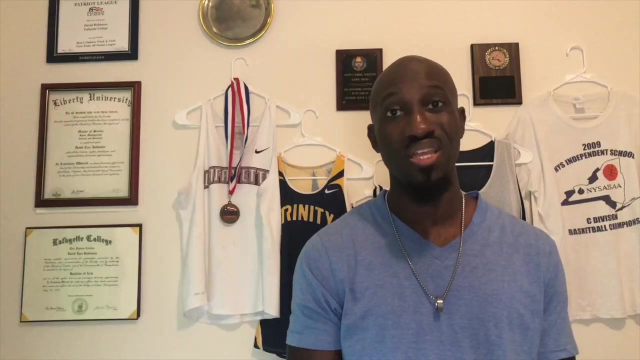 NAIA is often treated as the neglected stepchild of college athletics, but NAIA programs are often just as capable of providing everything that most NCAA schools can. If you are a recruit who is serious about getting college sports offers, it might be a mistake to spend too much time overlooking the NAIA. Thank you so much for watching this video.